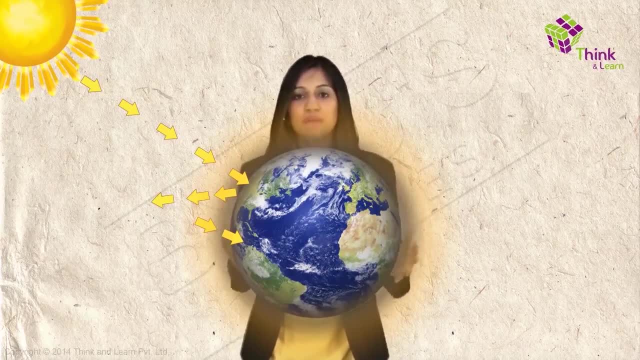 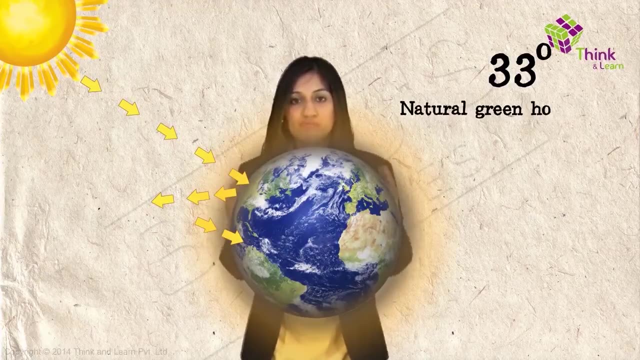 kind of trapping heat like a greenhouse does, keeping the planet at about 33 degrees hotter than it would otherwise be. This is called a natural greenhouse effect. It's a good thing, because without it the Earth would be way too cold. It would not be able to. 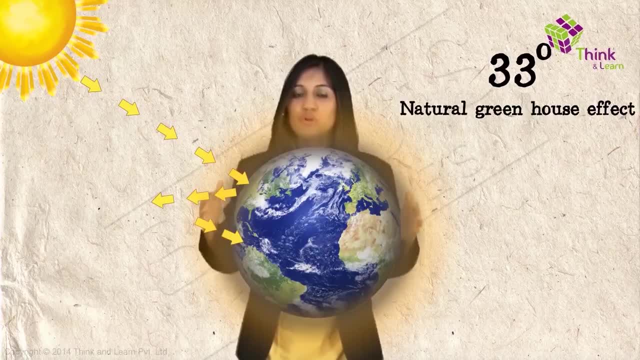 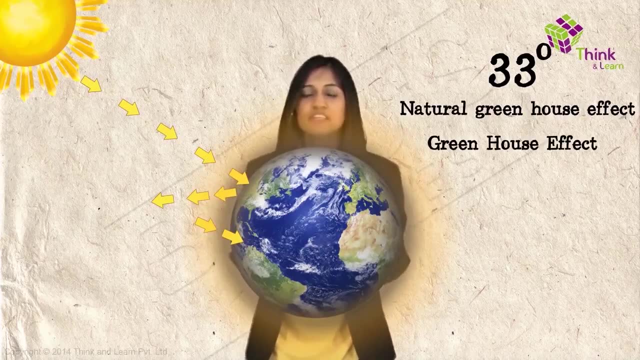 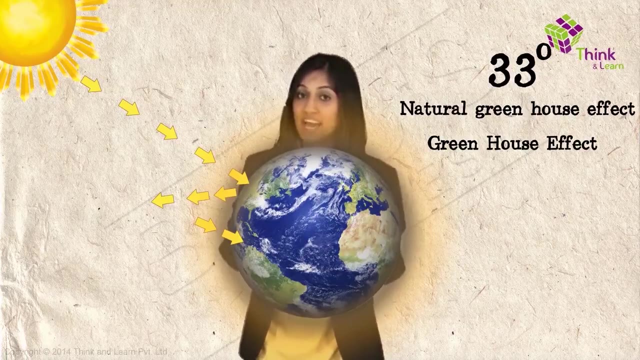 support the huge diversity of life on it. So this whole special phenomenon has an evil, special name. As you might have guessed, it's called the greenhouse effect. Now, greenhouse effect is good, just that too much of it is bad. And the bad kind of greenhouse effect is called the enhanced 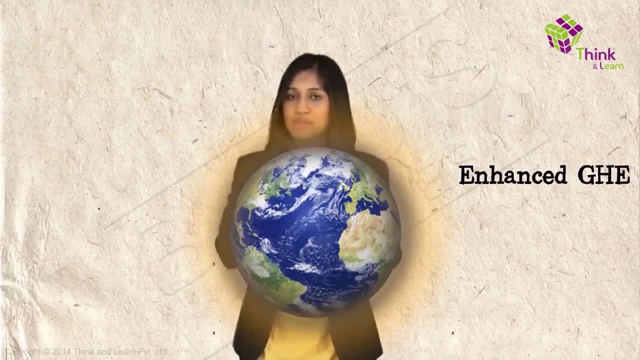 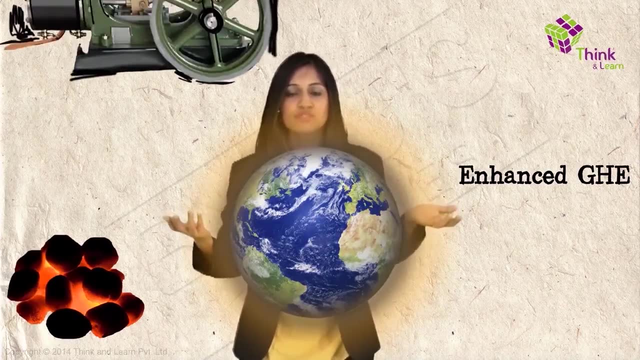 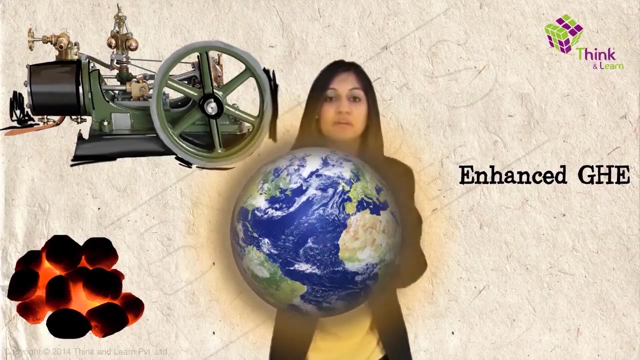 greenhouse effect. So what happens over here, You might already be guessing right. So we had this industrial revolution in the 18th and the 19th century, when coal-burning steam engines were first used. So humans have been using energy in far greater quantities. Car engines, for example, work by burning petrol. 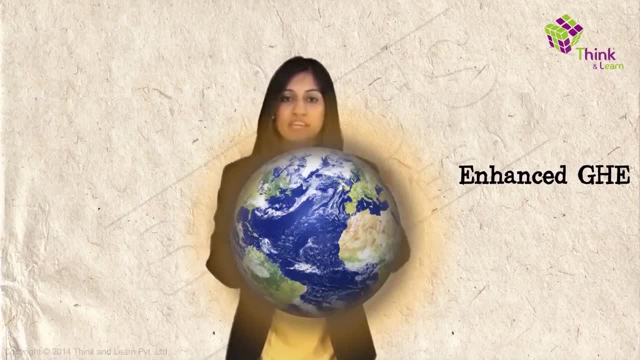 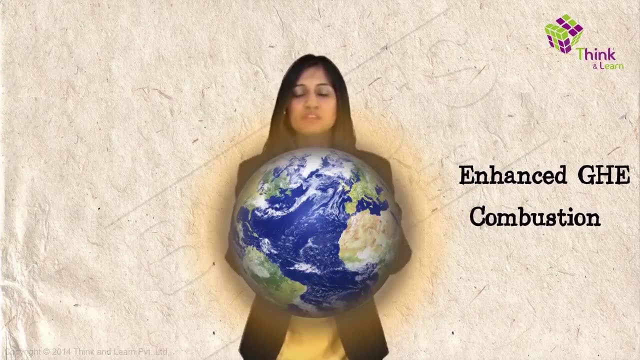 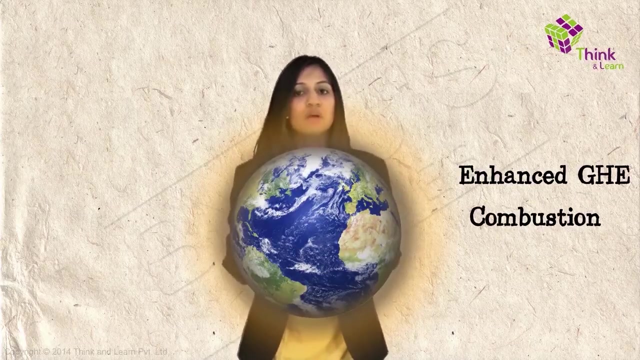 or diesel with oxygen in the air, make heat in a chemical reaction. You know this. it's called combustion And as a byproduct, combustion gives off invisible carbon dioxide gas, the same gas that our bodies actually breathe out. We discard it In a similar way these power plants use. 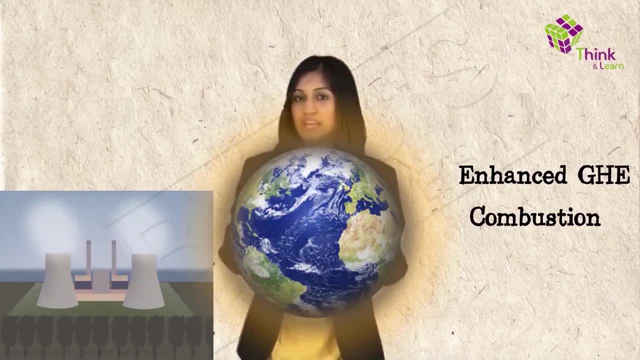 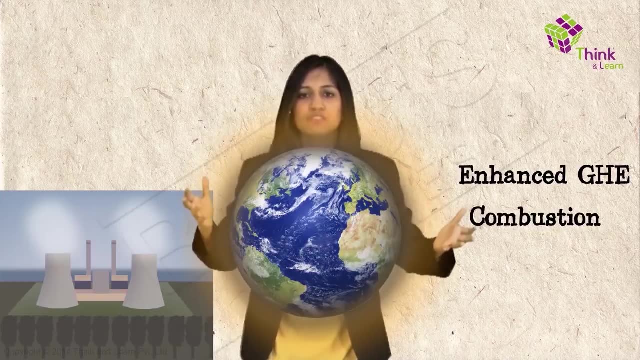 combustion to make electricity, you know, by burning fuels like coal and gas and oil. So they also give off carbon dioxide. So there's a lot of carbon dioxide being produced, huge clouds of them being produced in the environment, And all of these are called. 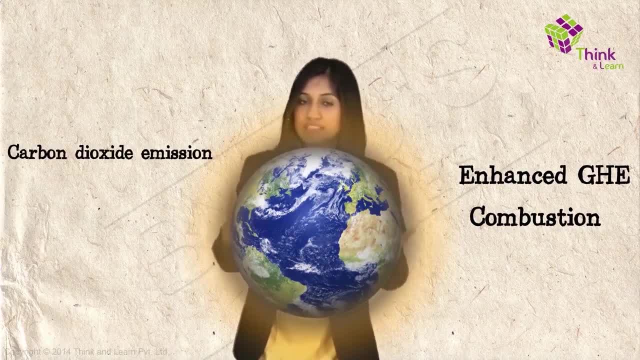 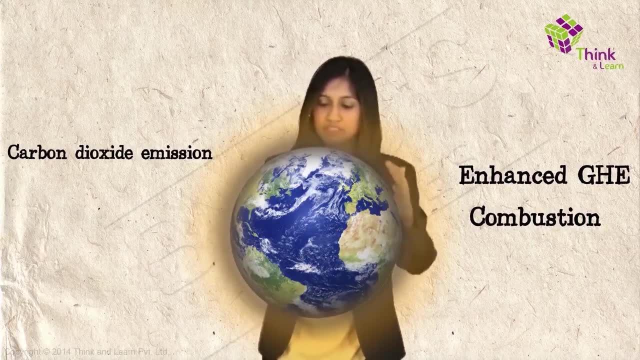 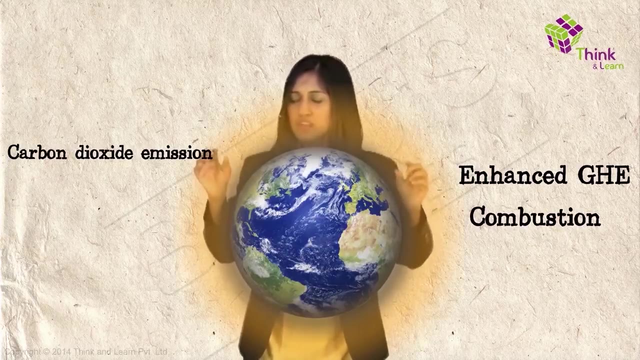 carbon dioxide emissions. What is coming out of the gas engines, what is coming out of the industries, all produced from burning fossil fuels. Now what happens is this excess carbon dioxide drifts up to the atmosphere, makes the earth's greenhouse gas just a little bit. 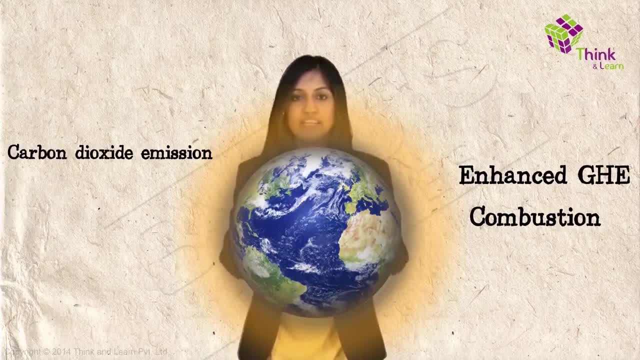 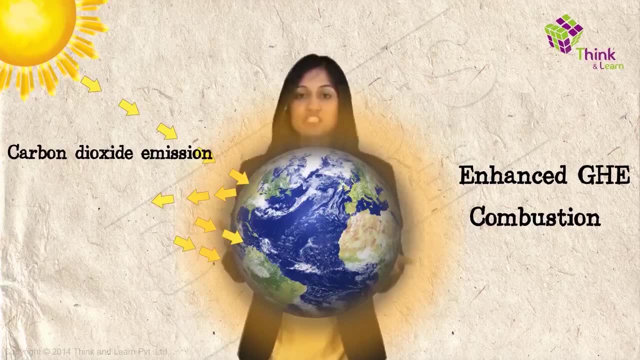 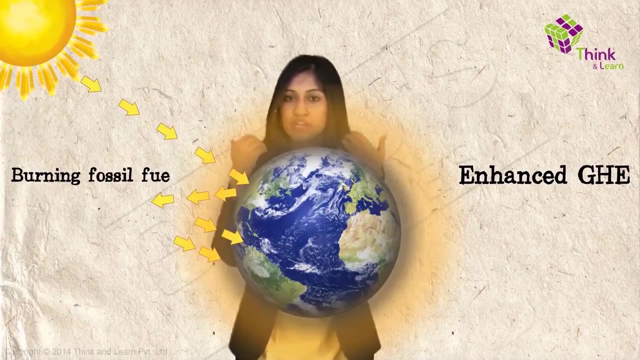 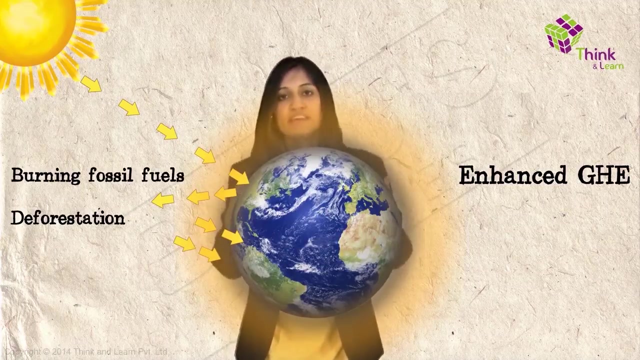 thicker. This is called enhanced greenhouse effect And, as a result, more of the sun's heat gets trapped inside the atmosphere. The planet starts to warm up. So this is summarize this whole thing. Burning fossil fuels gives off carbon dioxide. Deforestation reduces the number of plants available to take in that.